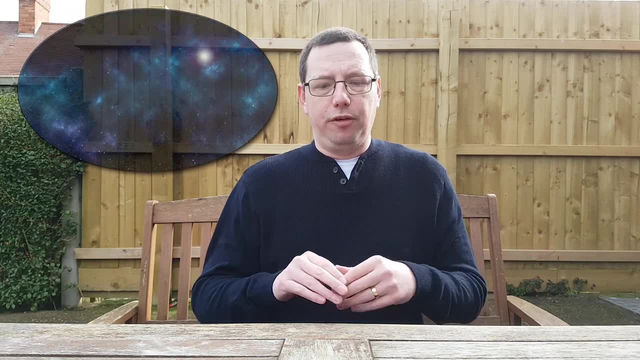 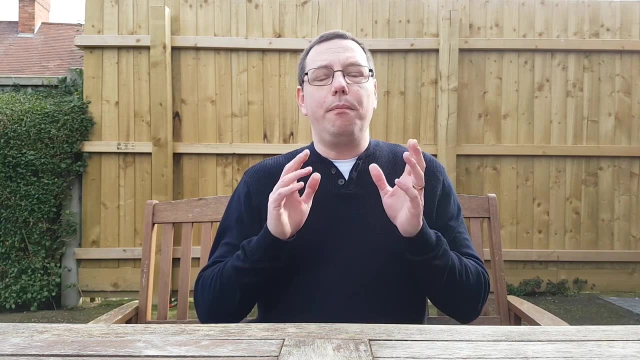 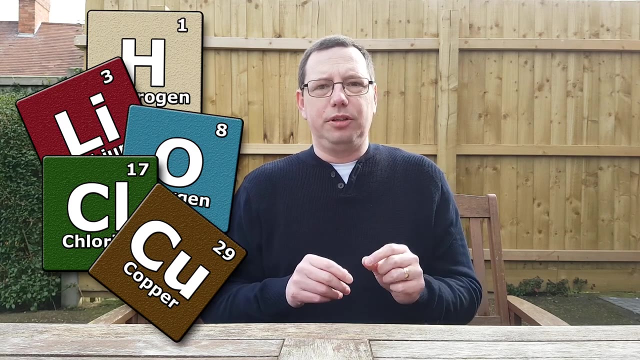 the building blocks that make up everything in the universe, From this table to me, to the camera that I'm filming this video on. everything is made of atoms. There are many different types of atoms. Each has its own name. We call these elements And these elements. 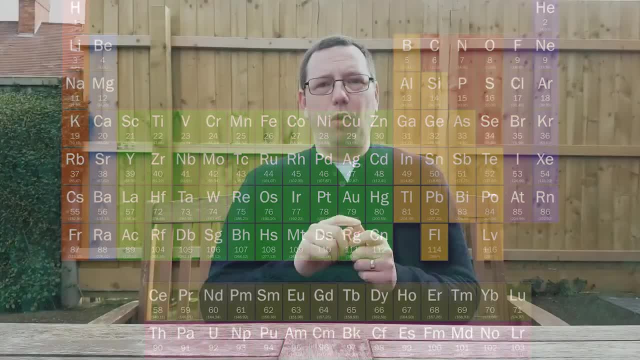 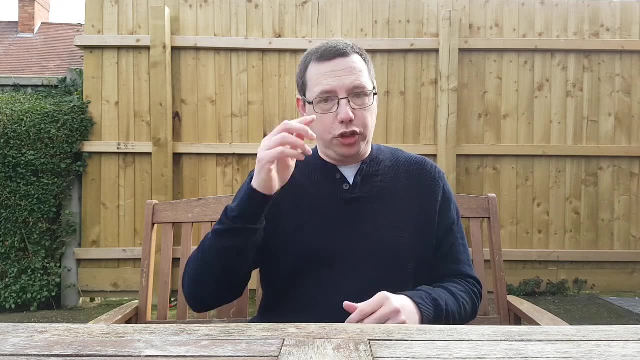 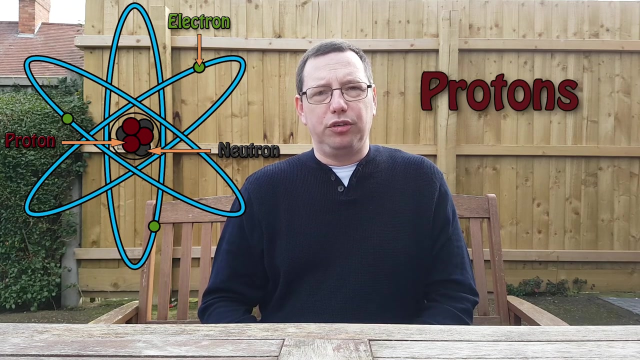 are organised on the periodic table, which we will be focusing more on in the next video. Atoms are incredibly small, Many, many, many thousand times smaller than human hair. Even though atoms are incredibly small, they are made up of three even smaller particles: Protons. 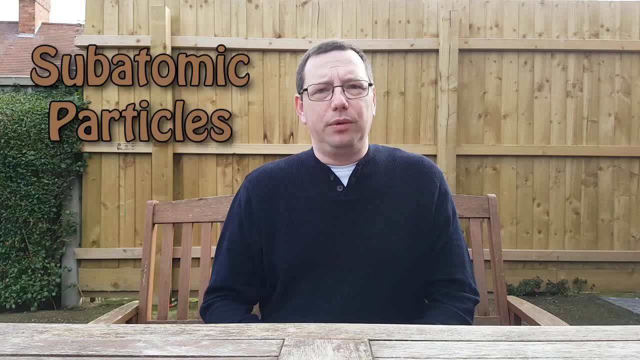 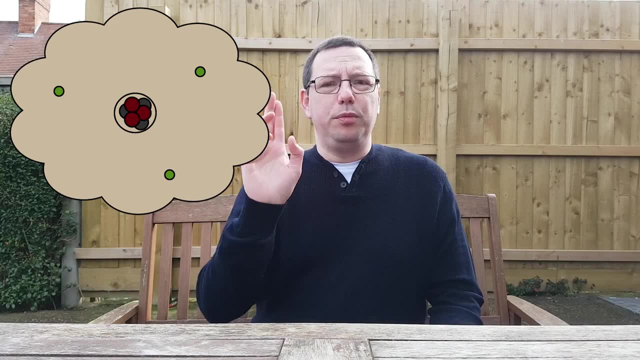 neutrons and electrons Together. these are collectively known as sub-atomic particles. The protons and neutrons are located in the centre of the atom called the nucleus. The electrons move around the nucleus in a type of cloud that contains shells and orbitals. 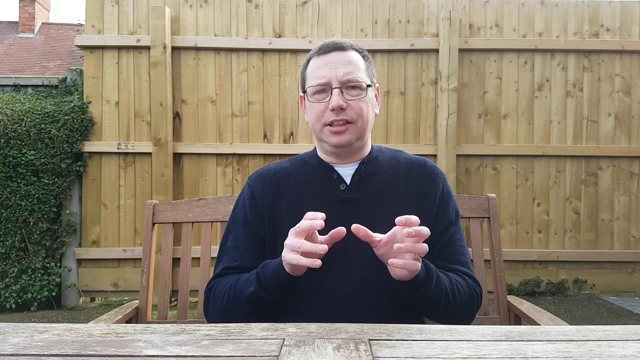 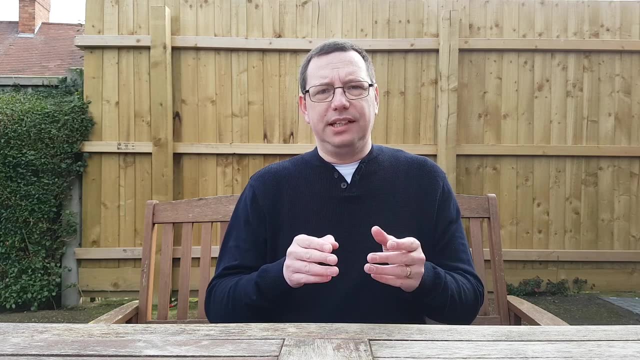 They are positively charged And the number of protons that the element has determines which element it is. If it's got eight protons, it's oxygen. Eleven protons, sodium. Seventy-nine protons, it's gold. We'll build more on this in the next video. Neutrons are neutral. They 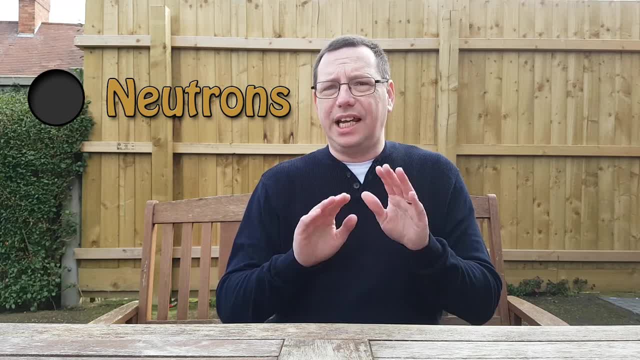 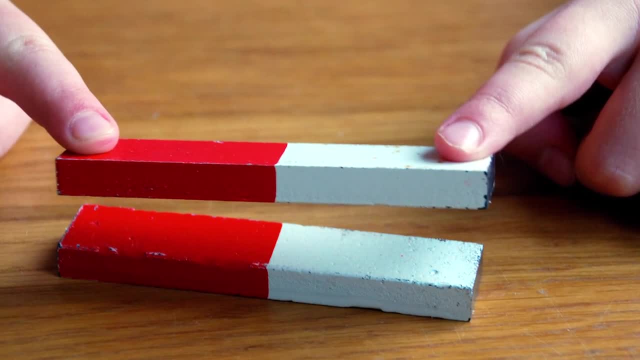 don't have any electrical charge, But they are important for keeping the atoms stable. Protons basically don't like being near each other. The positive charges repel each other, Much like when you get two magnets and you put them together: they just won't go together. 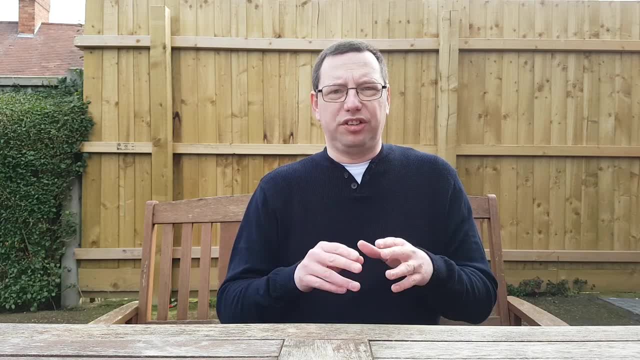 The neutrons are like the caretakers of the atom. The neutrons are like the caretakers of the atom. The neutrons are like the caretakers of the atom. The neutrons are like the caretakers of the nucleus: They keep the protons in line, Make sure they're on their best behaviour. 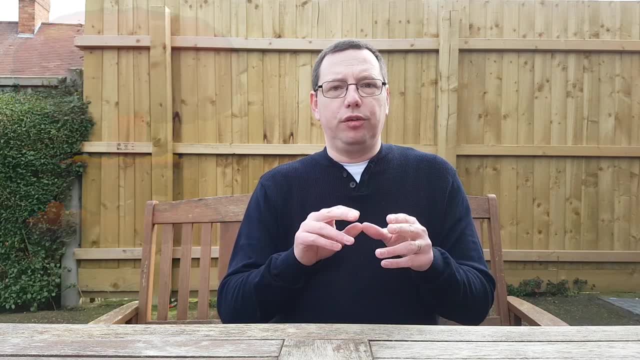 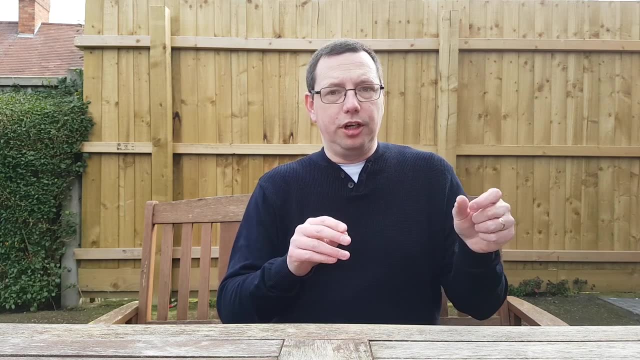 Without the neutrons, the atom would just tear itself apart. The more protons that the element has, the more neutrons that are needed to keep the atom stable Together. the protons which are positively charged and the neutrons which are neutral give the atom a positive 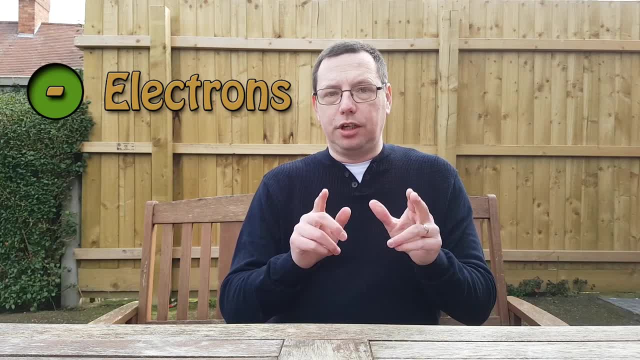 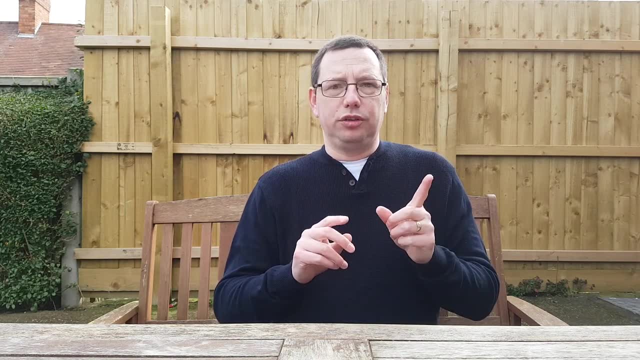 charge. Electrons, where all the interesting chemistry stuff happens, are negatively charged And are very, very tiny. compared to the much larger protons and neutrons. They're about 1800 times smaller. They whizz around the nucleus very, very quickly in.